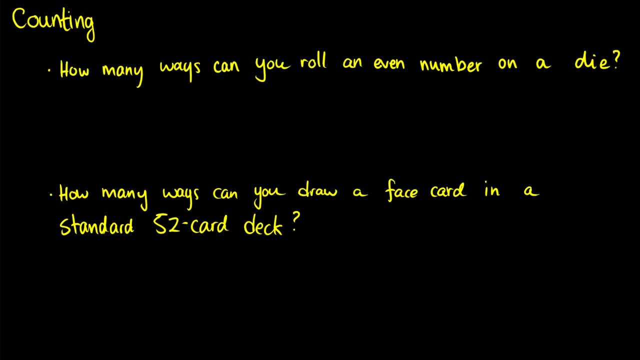 a very easy question: how many ways can you roll an even number on a six-sided die? So let's just specify this, that this is for sure six-sided. Well, which even numbers do you see on a six-sided die? You see the numbers two, four and six. Okay, so there's three different ways. 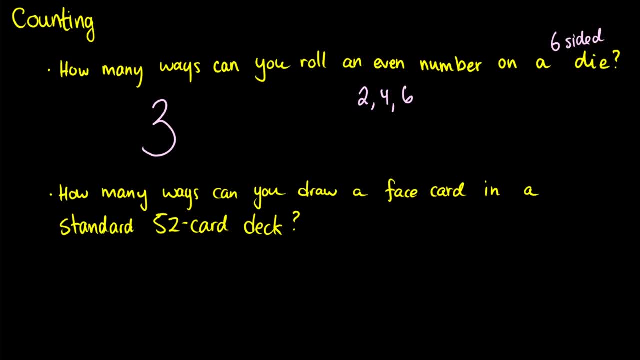 that we can roll an even number on a six-sided die. Okay, easy question: How many ways can you draw a face card in a standard 52 card deck? Well, what is a face card? A face card is any of the jack queen or king And, of course, for each of these jack, queen and king. 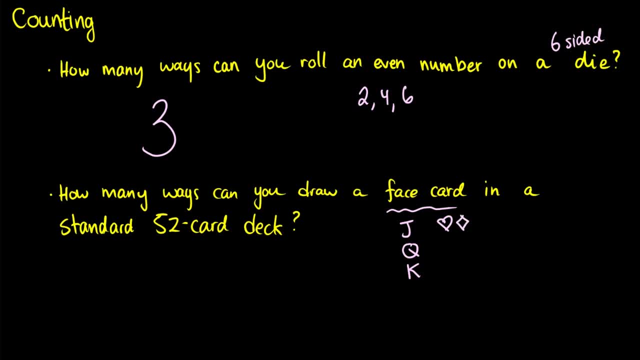 we have four different suits: We have hearts, we have diamonds, we have clubs and we have spades, all of which I am not going to draw. So in total we have 12 different ways that we can draw a face card from a standard 52 card deck. There's four jacks, four queens and four kings. 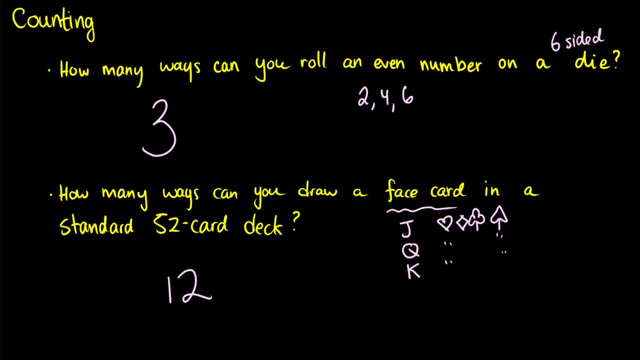 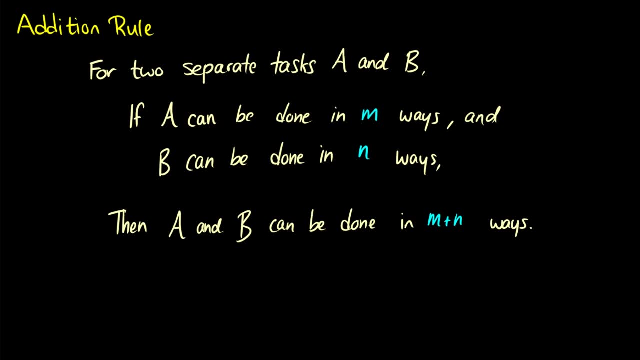 Okay, so this is just doing one task inside of some specific domain. We have this thing called the addition rule, And this is when we have two different tasks, A and B. So we could say that A is rolling an even number and B is picking a face card. 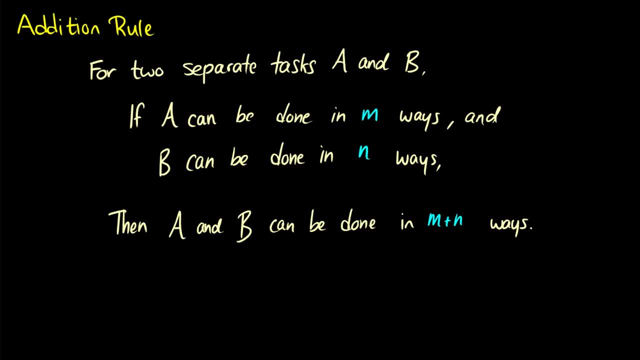 Okay, so let's say that task A can be done in M ways and task B can be done in N ways, Then task A and B can both be done in M plus N ways, And these are when the tasks are separate. So if we go back to that original example, 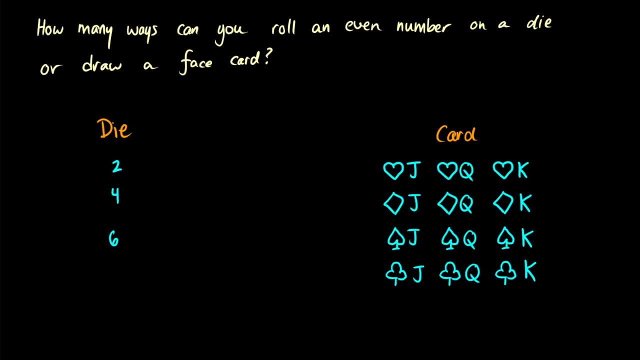 we could say: How many ways can you roll an even number on a die or draw a face card, In which case we have our task A, which is rolling an even number. There are three ways to do that. Then we have our task B, which is to pick a face card from the deck. 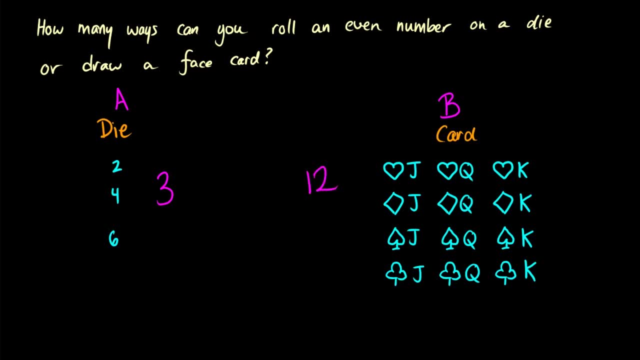 And there are 12 ways of doing that. So when we say How many ways can you roll an even number three or a face card from a set of 52 cards, it would be 12.. We add them together and we end up with a grand total of 15 different ways to do either task. 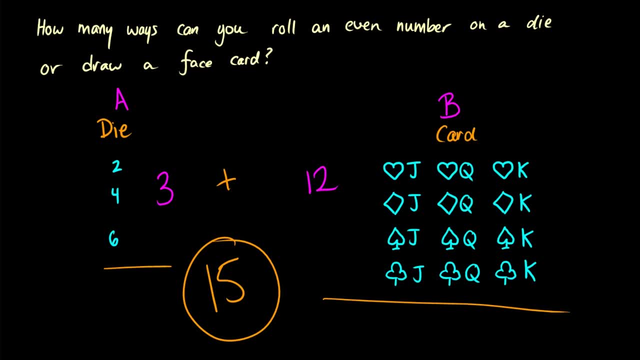 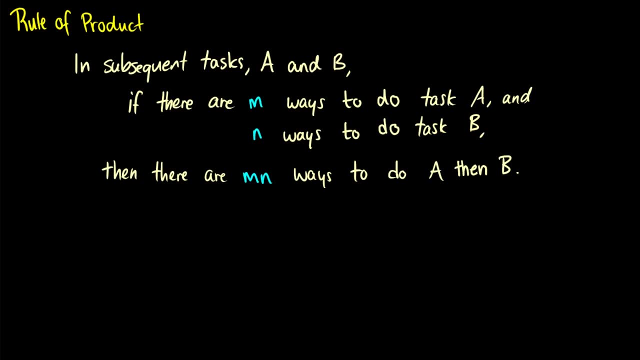 Either we get one of the even numbers or we get a face card from a deck. Okay, Now the rule of product is slightly different. We say here, with the rule of product, In subsequent tasks A and B, if there are M ways to do task A and N ways to do task B. 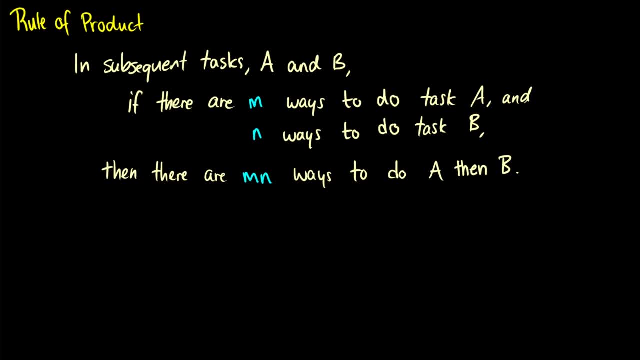 then there are M times N ways to do A, then B, In other words. other words, these are tasks that are done one after another. With the rule of addition, it's doing one task or another one. With the rule of product, it's doing them subsequently. So here's. 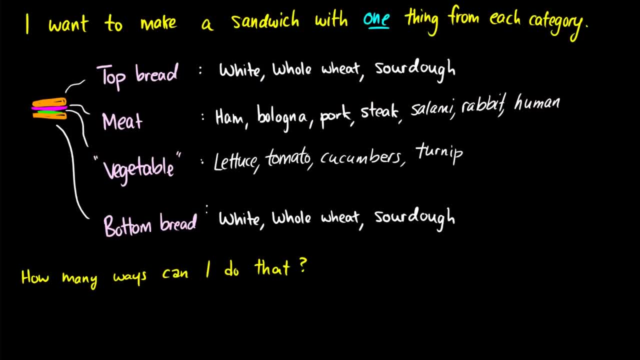 an example of a rule of product question. Suppose I want to make a sandwich and I have four different steps where I have to make choices. So I need one piece of top bread, which can be white, whole wheat or sourdough. I need one meat, So we have ham, bologna, pork, steak, salami, rabbit and human. 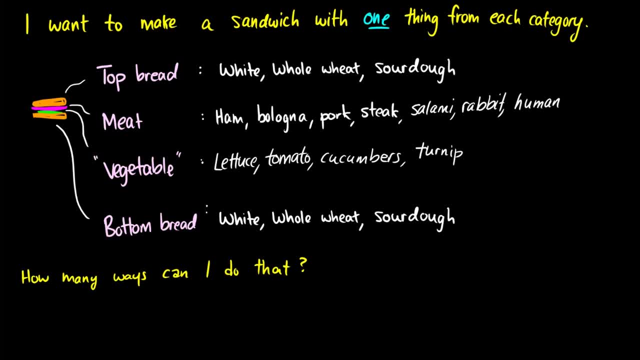 meat. We want some vegetable, So this could be lettuce, tomato, cucumbers or turnip, And we also have a bottom bread, which can be white, whole wheat or sourdough. We go wild here. The top and bottom bread can be different. So how many ways can we do that? Well, it's really like. 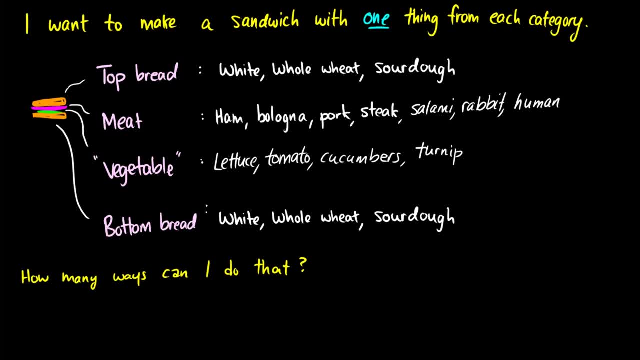 having four different tasks that are all done one after another. For instance, first we choose a top bread, Then we choose a meat, Then we choose a vegetable, Then we choose a bottom bread. So it's A, B, C or D. 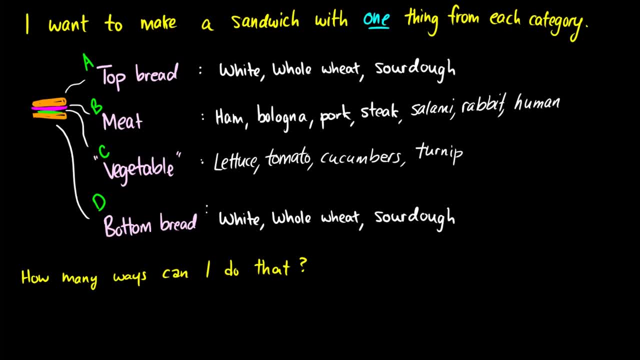 So four tasks. Well, for the top bread we have three different choices. Okay, For the meat, we have one, two, three, four, five, six, seven choices. So ham, bologna, pork, steak, salami, rabbit and human For vegetables. 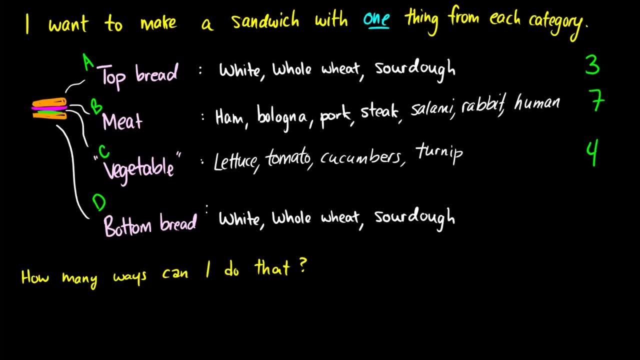 we have four choices And for the bottom bread, once again we have three choices, And when we're doing subsequent tasks we need to multiply. So there's three ways to do task A, seven ways to do task B, four ways to do. 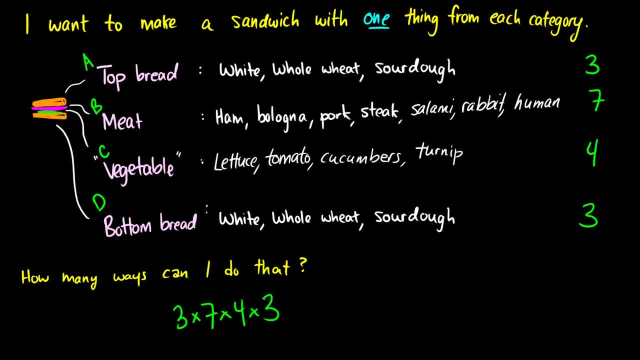 task C and three ways to do task D. In other words, in total there's going to be 21 times 12 different ways, which should be something like 210 plus 42, which is 252 ways in total. So there's 252 different. 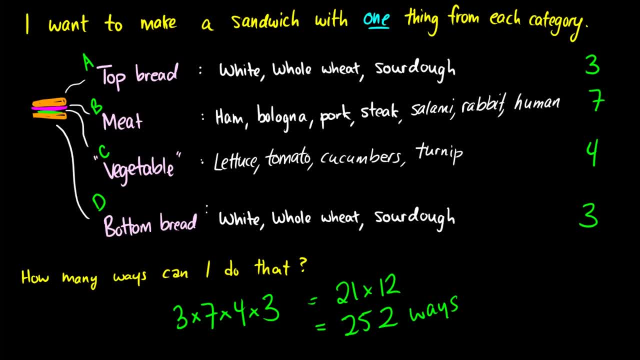 sandwiches we can make. Okay, so to go over that logic again, essentially we're picking one from each, So we might pick white bread on top, bologna as the meat, lettuce as the vegetable, and then whole wheat as the bottom bread. 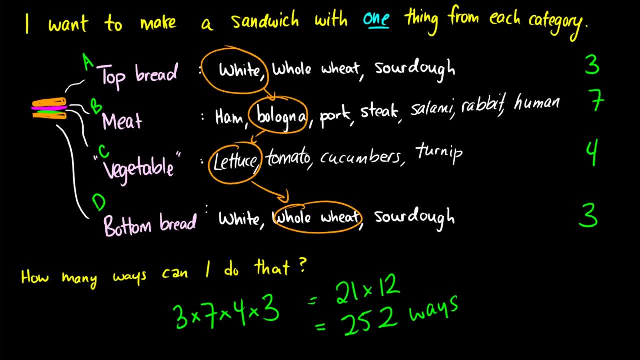 Okay, so in the first task, we pick one way to do it. The second task, we pick a second way. The third task, we pick a third way and we get 252 total options. So that's an example of the rule of product. 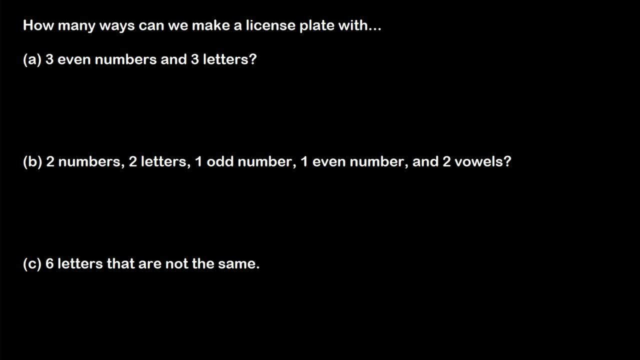 Okay. so let's put this into an application, let's say making license plates. So where I'm from, license plates consist of six symbols. three of them are numbers and three of them are letters. So let's say we have some restrictions on the types of things we can put on our license plates. So, for example, we want our numbers to just be three even numbers and then we want three letters. Okay, and we're not going to be too specific about where these letters and numbers show up. They just have to show up as a comment step. 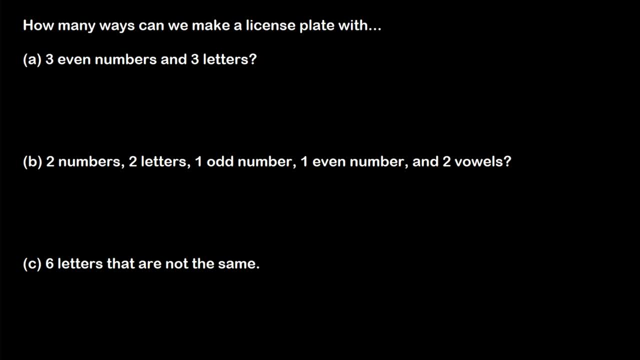 Okay, So we don't have to do a few things to be specific about where these letters and numbers look. We want to sort of have spooninum here and we're going to put just a few numbers into what we're motivating the tab. So we have utilise this. the order of the starters. we want to have PossFA. 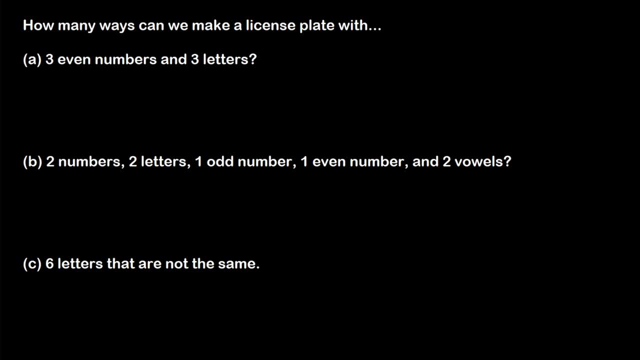 Thank you for listening and have a good rest of the week. Have a great rest of the week everyone. And we're not going to be too specific about where these letters and numbers show up. They just have to show up somewhere. So three even numbers. 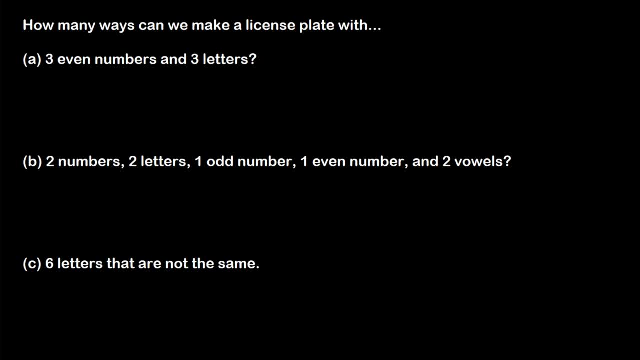 Well, the even numbers between 0 and 9 are 0,, 2,, 4,, 6, and 8.. So for each of the even number spots we have five different choices. So we have five ways to pick the first number, five ways for the second and five ways for the third. 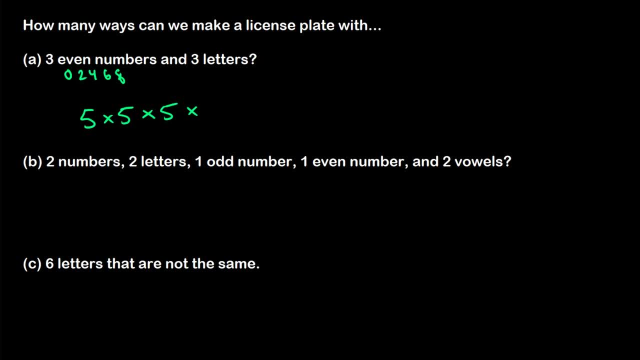 Now for the letters. well, there's 26 different letters in the alphabet. We can have 26 letters for our first choice, 26 letters in the second choice and 26 letters for the third choice. So in the end we have 5 to the 3 times 26 to the 3 different license plates that we can make. 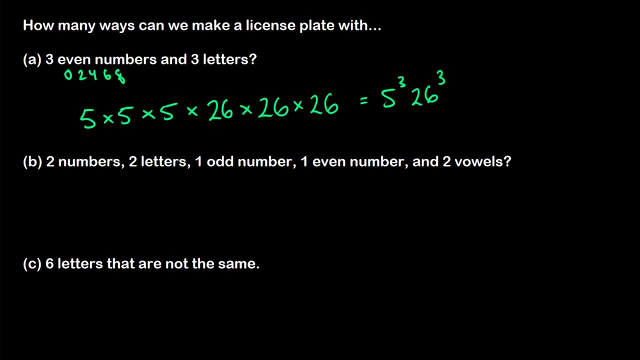 Okay, so that's a lot of license plates. Now what if we restrict ourselves in a different way? Okay, so let's do an 8-symbol license plate. So first I have to have two numbers. Well, there's 10 numbers to choose from, 0 through 9.. 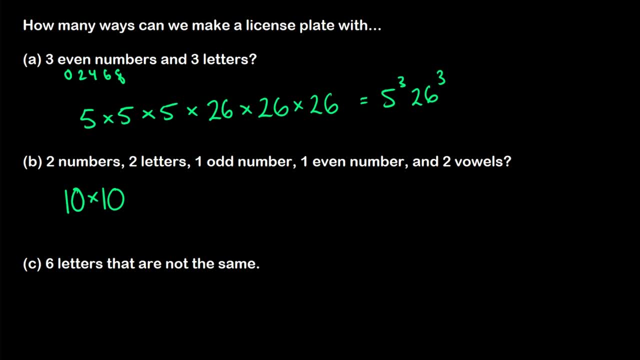 So we have 10 choices for our first number, 10 choices for our second number. We have two letters, so we need two cases of 26 choices here, One odd number, so we have 1,, 3,, 5,, 7, and 9.. 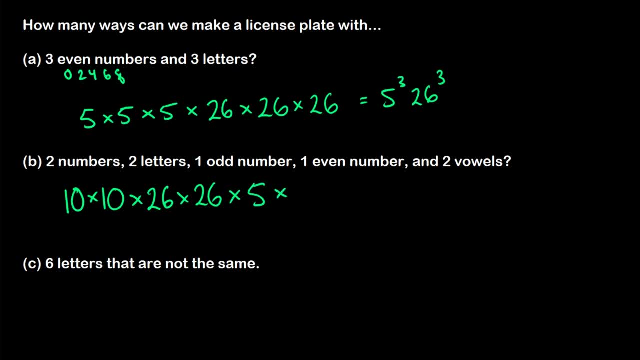 That's five choices, One even number 0,, 2,, 4,, 6,, 8.. Five choices And then two vowels. So we have A E I O U. So we have five choices for each vowel. 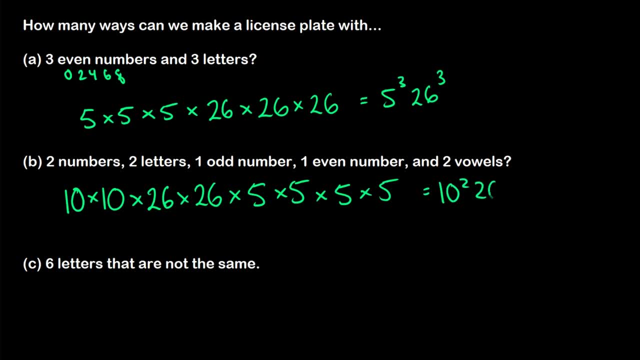 So what we end up with is 10 squared times 26 squared times 5, to the 4 different ways of making this license plate. Okay, so two numbers was our 10 by 10.. Two letters is our 26 by 26.. 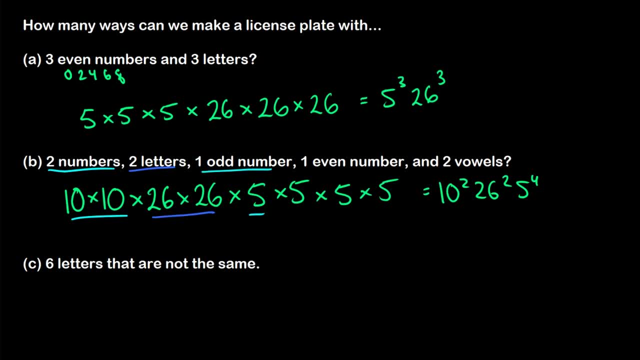 One odd number is our multiplying by 5 cases. We have one even number, Five cases each as well, And then our two vowels are each five cases. So we can see how these numbers line up. Okay, now here's a more interesting question. 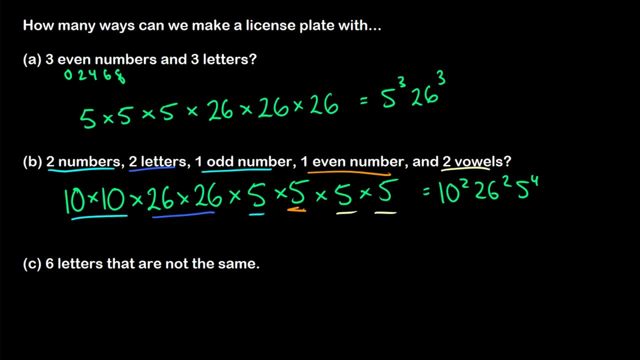 How many license plates can we make that consist of six letters where they're not the same letters? Okay, so this means let's simplify this first. If we have, say, four letters we're choosing from and we're going to make a two-letter license plate out of these four where we can't reuse the same one, 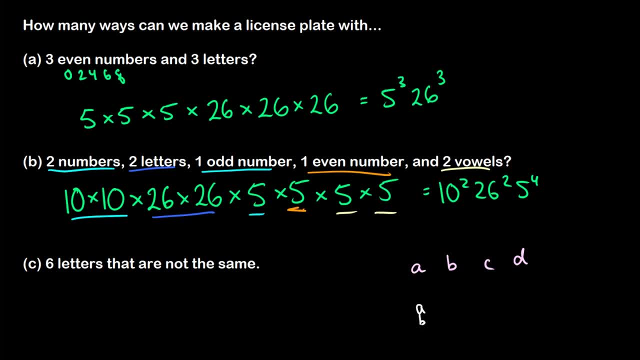 let's say, for our first spot we could pick A, B, C or D. That could be our first spot. Well, if we pick A, then we can no longer pick A for our second slot. So really, for our first slot, we have four choices that we can choose from. 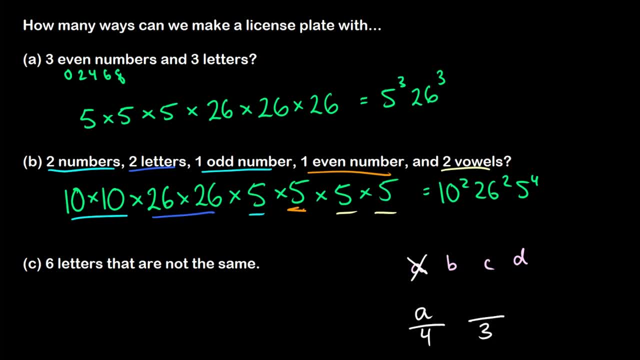 With our second slot, because we can't pick A. we only have three choices left. So if we're working with just four letters and we want two spots, our solution is going to be four times three. So if we have six letters that are not the same, 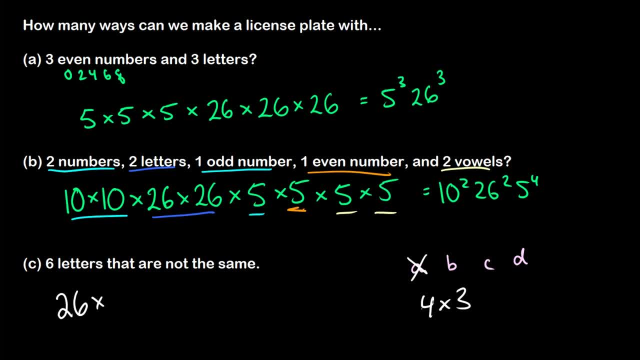 then, for our first slot we have 26 choices, And whatever letter we pick we can't reuse. So for our next slot we have 25 choices. for the second slot, 24. for the third slot, 23. for the fourth slot. 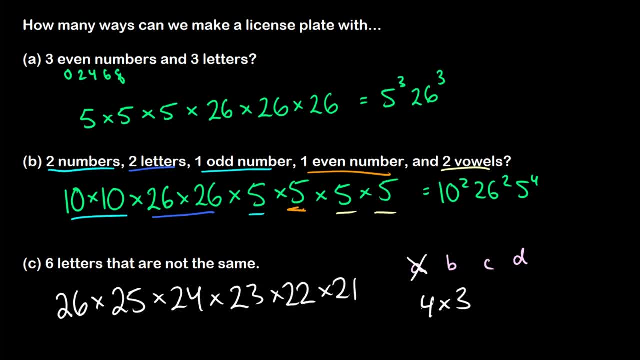 22 choices for the fifth slot and 21 choices for the final slot. So this is how many license plates we can make where the letters are not the same. So this is it for the rule of addition and for the rule of product.